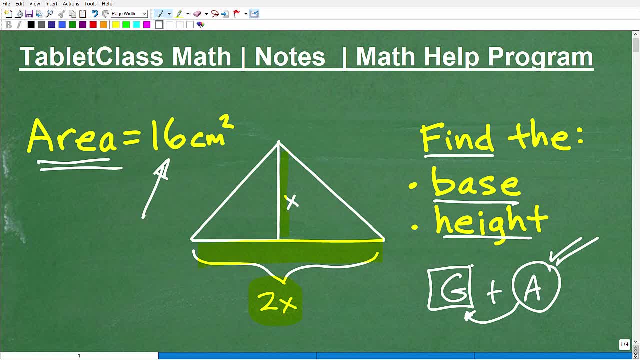 know a decent amount of algebra to do well in geometry. Now, as you're looking at this, if you think you know how to do it, I would certainly encourage you to pause the video and go ahead and see what you can come up with, But of course, I'm going to solve this here in 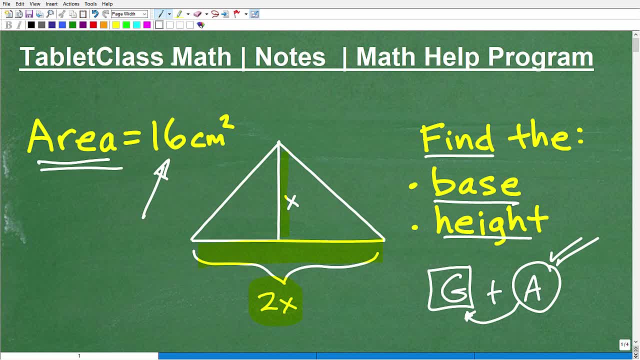 just one second, But first let me quickly introduce myself. My name is John. I'm the founder of Tablet Class Math. I'm also a middle and high school math teacher And over several years I've constructed what I like to believe is one of the best online math help programs there is. 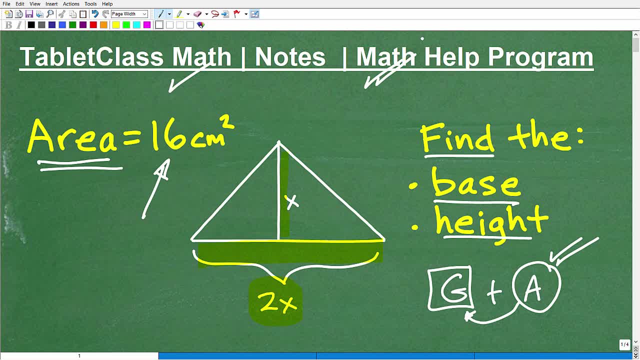 Of course, I'll let you be the judge of that. You can check out my math help program by following in the description of this video. But basically I have 100 plus different math courses, ranging from pre-algebra, algebra 1, geometry, algebra 2.. These are all very comprehensive, thorough courses and 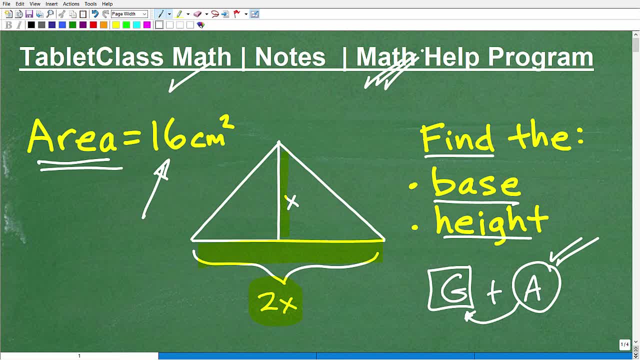 nothing with no small tutorials. I mean these are complete comprehensive courses, proven courses as well. I'm going to be launching pre-calculus here shortly And I also do a lot in the area of test preparation. So if you're studying for the GED, SAT, ACT, 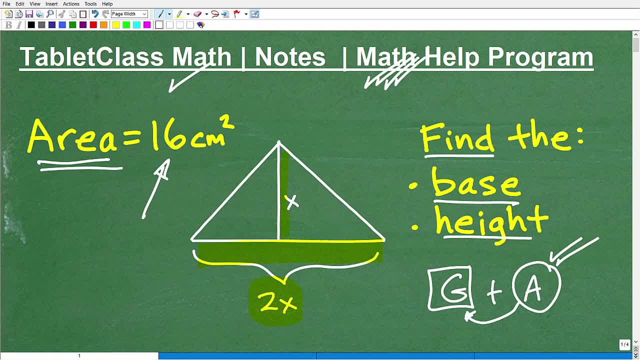 maybe the GRE, GMAT, CLEP exam, ALEKS exam, ACCUPLACER teacher certification exam, nursing entrance exam. there's a ton of reasons why people study math outside of a math course: because you're taking these exams, which have a pretty significant amount of math on them. 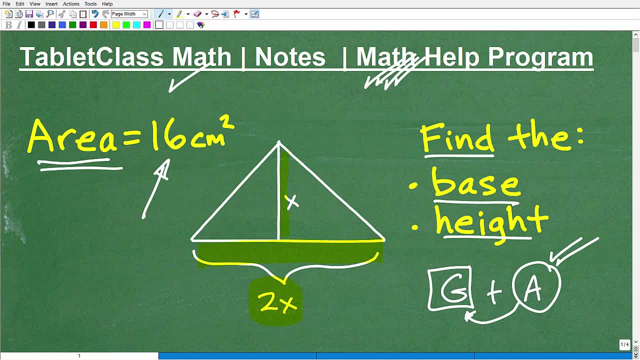 And if you don't do well in the math section, you don't do well on the exam. Of course, we don't want that to be the case. So if you're studying for a particular exam, just go to my site. check out my full course catalog. I should have what you need. 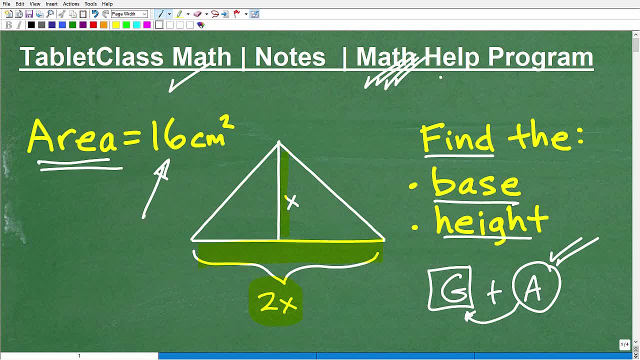 If I do not, please drop me a line and I'll help you out the best I can. I also do a lot with independent learners, like homeschoolers, have a great homeschool learning program and then obviously help those of you that are struggling in your current math courses. 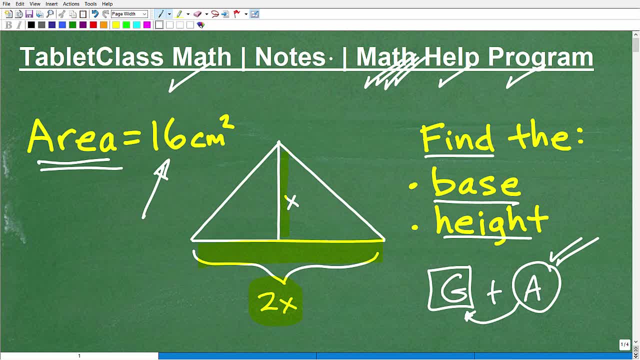 Now, one thing I cannot do for you that you must do for yourself if you're serious about really learning math, that is taking notes. You got to take great math notes. So over decades of teaching math, one thing is apparent to me: that those students who take excellent math notes 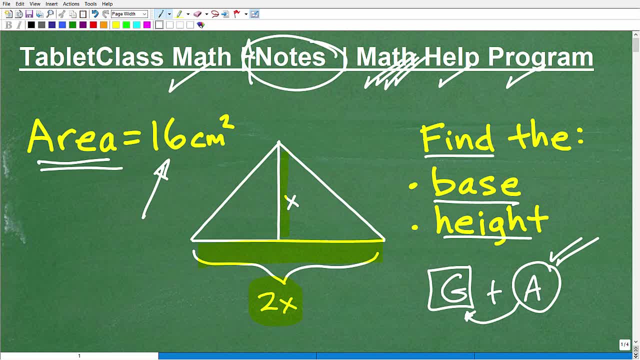 almost do excellent in their grades and their tests and their quizzes, et cetera, et cetera. And the reverse is true: Those students who are, like myself, way back in the 1980s, highly distracted, talking to my friends, thinking about the weekend. 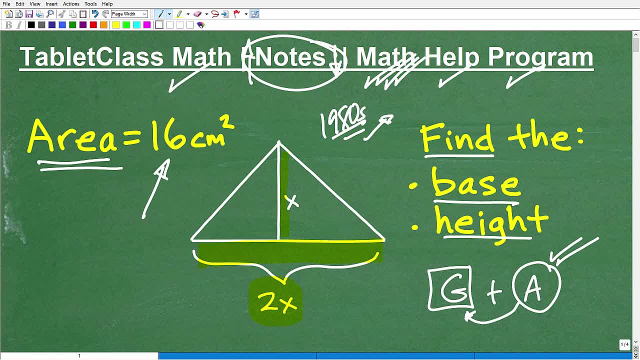 just kind of pretending to do stuff every time the math teacher looked at me. Listen, I didn't get serious about becoming a student until I went to college. Well, that was after the Marine Corps. But basically you need discipline to do well in your studies. 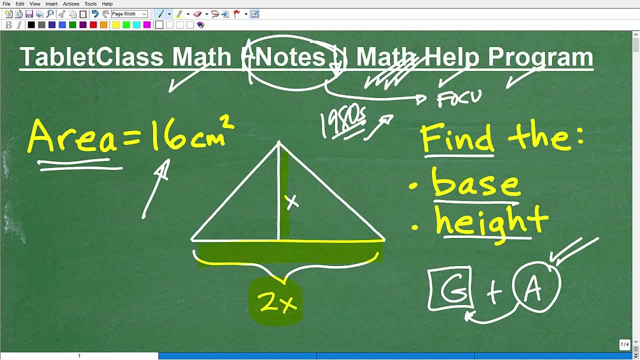 Because discipline is what's required for you to focus And no other activity is better than note-taking to help you focus in class. So if you want to kind of get a good sense of how well you've been paying attention in your current class, look at your notes. That's a pretty good. 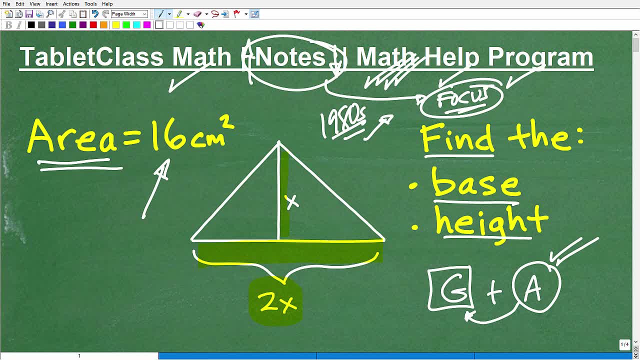 reflection, So improving your note-taking. in the meantime, if you need something to study, from which of course you do, I offer detailed, comprehensive math notes to include pre-algebra, algebra one, geometry, algebra two and trigonometry. You can find the links to: 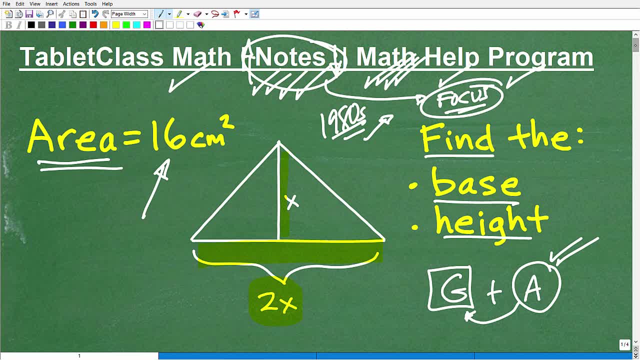 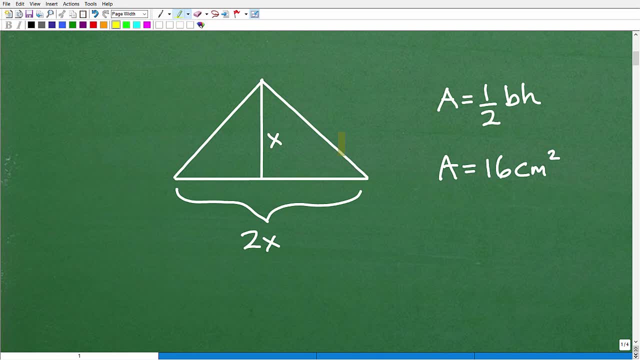 those notes in the description of this video. Now let's go down here and check this problem out from this perspective. So here is our given information. Okay, we have this triangle, We know that this is the base, This is the height And we know that the area is 16 centimeters. 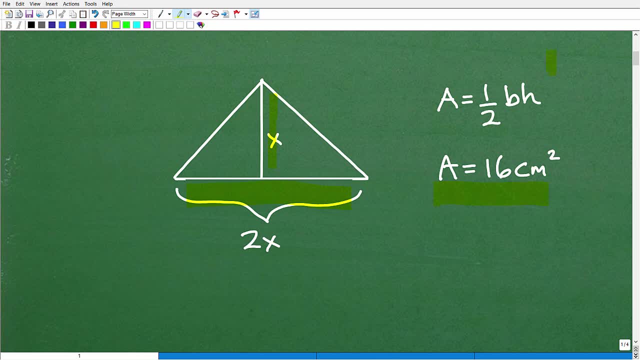 square. But we need one more piece of the puzzle And that is the formula. Okay, the formula for the area of a triangle. So the area of a triangle is equal to one half base times the area of a triangle Height. So 2x here is our base And x- okay, this is our height And we know the area, So we can. 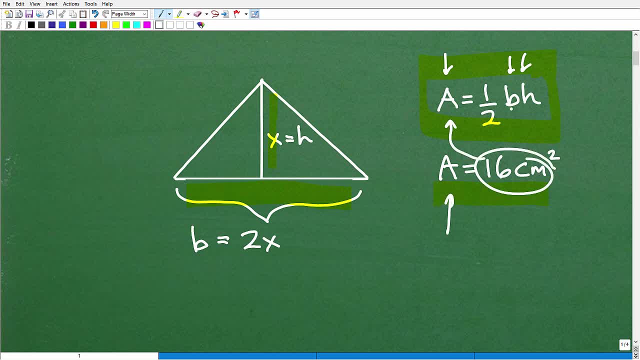 plug in this information right here. Okay, we know what our base is. Of course, that's that We could plug in right there And we could plug in our height information into this equation and solve. So this is the setup. Now, if you think you know what to do from this point forward, 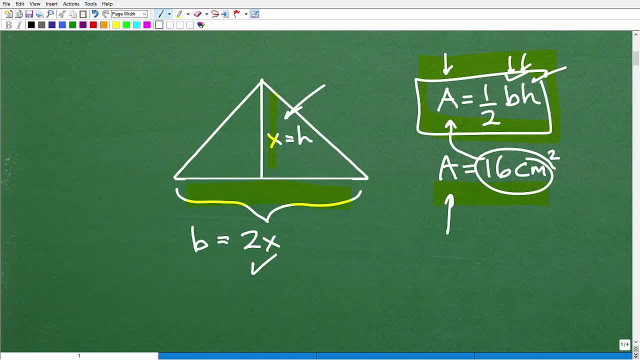 definitely go ahead And give it a shot, Pause the video and see what you can come up with, But this is basically basic algebra here. Okay, so we have the information. that kind of told you what's required to solve for these particular- the base and the height. But let's get into it now, Of course, 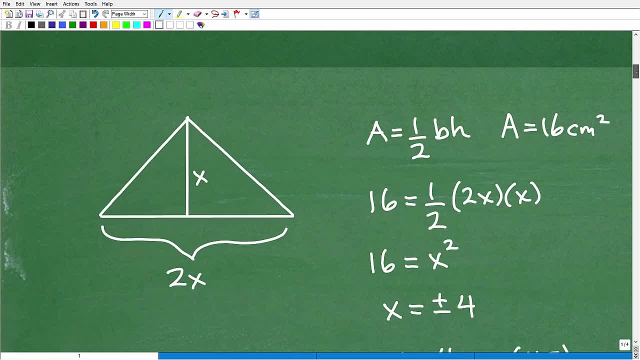 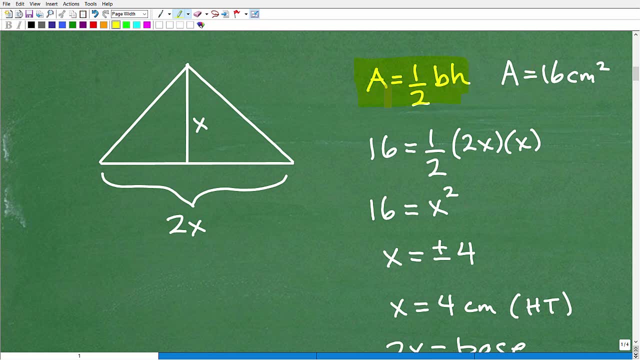 pause the video if you don't want to see the solution, but I'm going to show it to you right now. Okay, so here's the formula that we need: Area equals one half base times height. So what is our area? And we know that this is the area. So we're going to plug in our area And we know. 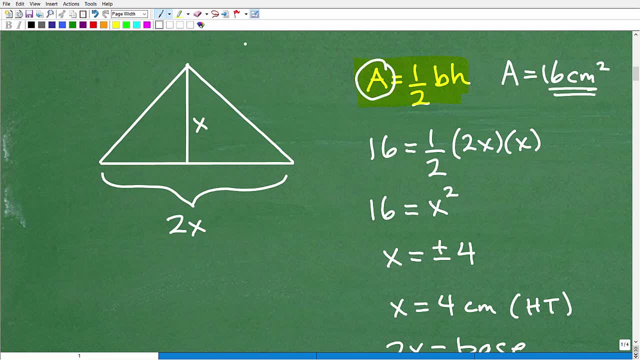 that this is our area. Okay, well, it's given to us 16 centimeters squared, but we'll just plug it in as 16.. We can kind of skip the units of measure right now. We'll deal with that at the end Then. 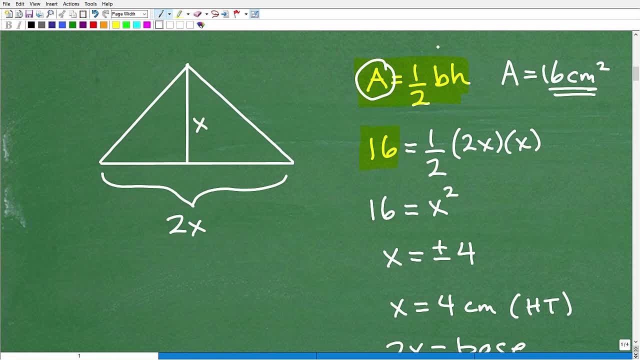 we have one half Okay, base, Okay, what is the base? again, The base is 2x, Because that's what I'm plugging in right there. That's my base, And then my height is x. All right, so this is the. 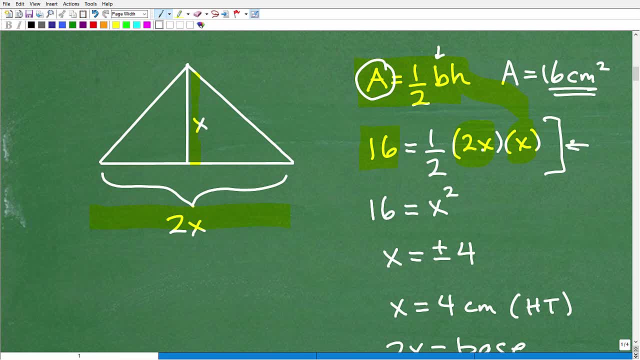 setup that you need to have constructed. Now. if you did this, if you got this right, then that's excellent. All right, I'll give you a little smiley face for that, especially if you already knew the formula to use. So that's very, very good. Now, from this point forward, we're talking about basic algebra. 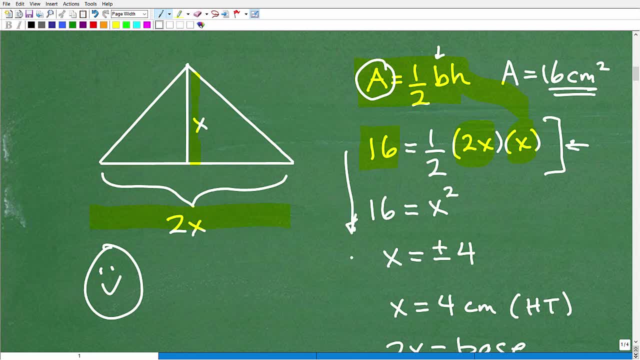 So if you're struggling with this stuff, you need to review how to solve equations and algebra. That's a huge topic, So you know, I encourage you to check out my videos on my pre-algebra and algebra playlist, Of course, if you're really really serious about all of this, definitely. 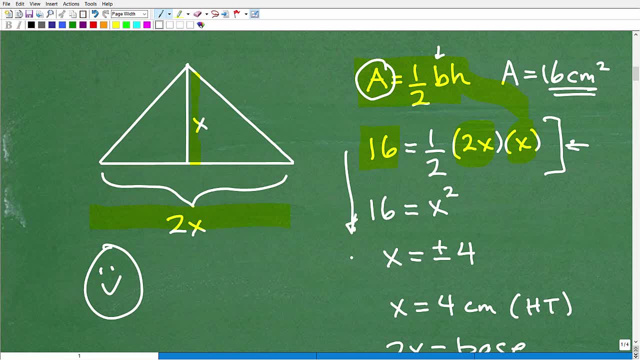 check out my courses. If you're in geometry, I have a great complete geometry course. Of course you may need algebra to be ready for that course, But you know, let's get back to the problem, All right. So here we have one half times 2x times x. So this one half right here and this two will. 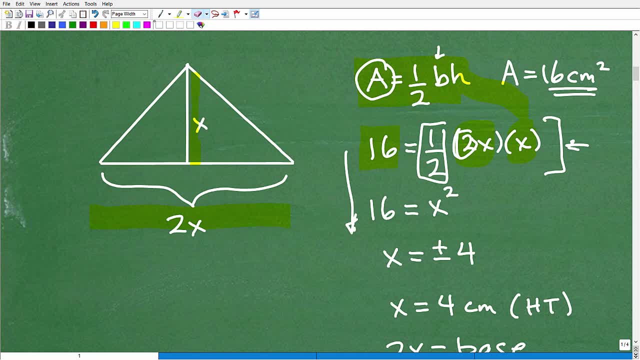 cross cancel. Matter of fact, let me just go ahead and show you this a little bit more thoroughly, for those of you that need to see this. All right, So this is the part that we're figuring out right now. So we're going to go: this number times this number One half times two is, of course, one. 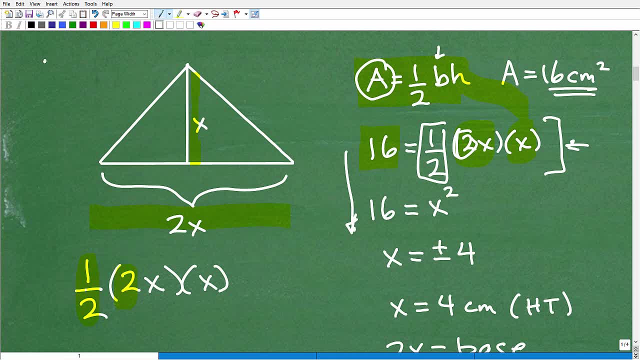 Okay, So that we could just in algebra we don't write one x, It's just x. Okay, So if you see an x or y, there's a one in front of it. So now I have to figure out what x times x is, and that is x. 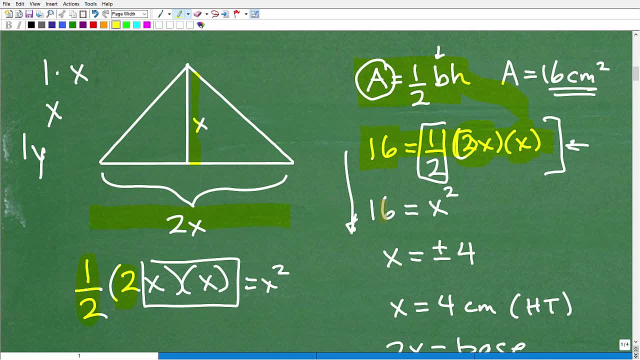 squared. So that's why here- okay, we get down to: 16 is equal to x squared. So how do I solve this basic equation right here? This is actually what we call a quadratic equation. But the way we solve this is: I have x squared, I want x. So if I take the square root of both sides, okay. if I take the 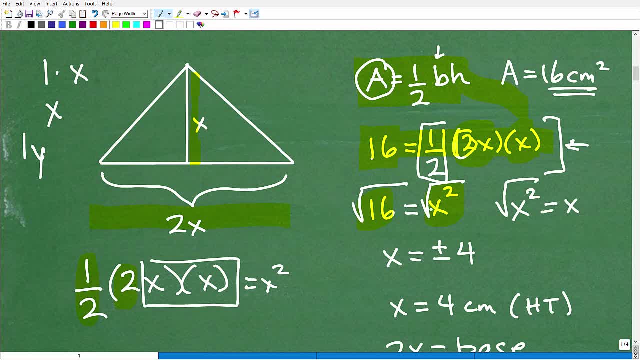 square root of an x squared. I get an x and that's what I want. So the square root of x squared is x. Okay, That doesn't make a difference on the left or right-hand side. Remember, the left is equal. 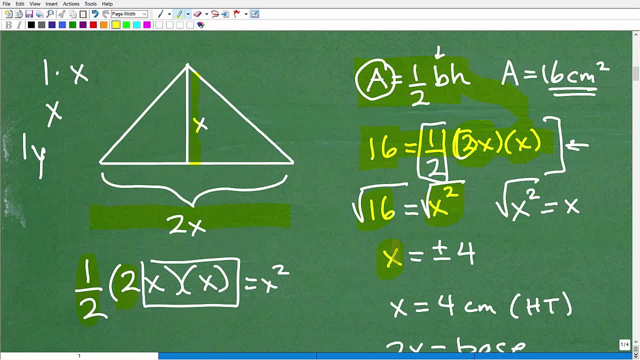 to the right. The right is equal to the left. So the square root of x squared is x and the square root of 16 is a positive and negative 4.. But let's throw out the negative here. We'll have a 4 and a. 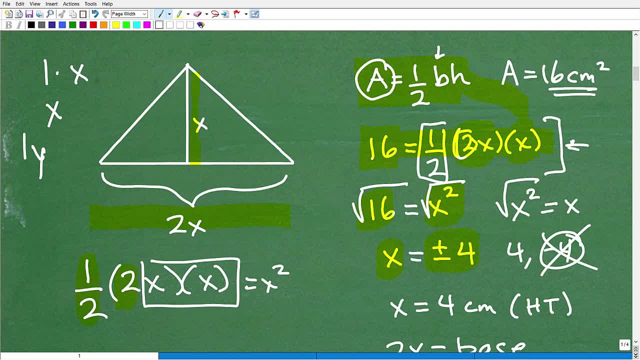 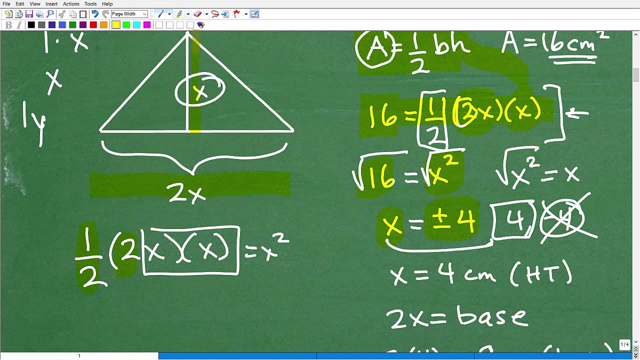 negative 4.. Let's throw out the negative 4.. Let's throw out the negative 4.. Let's throw out the this version or this answer, because we're dealing with measurements. okay, We're not going to have negative centimeters, So 4 is the correct answer. Okay, So x is equal to 4.. So what is x? Okay, Well, 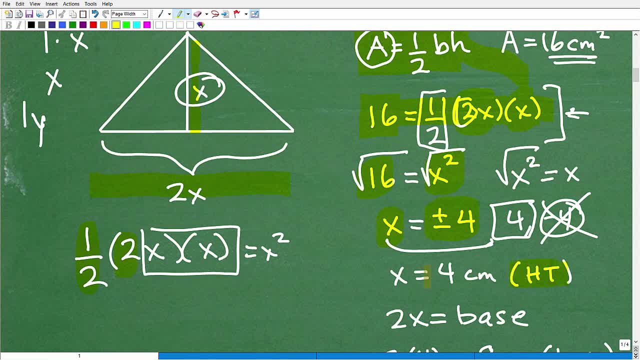 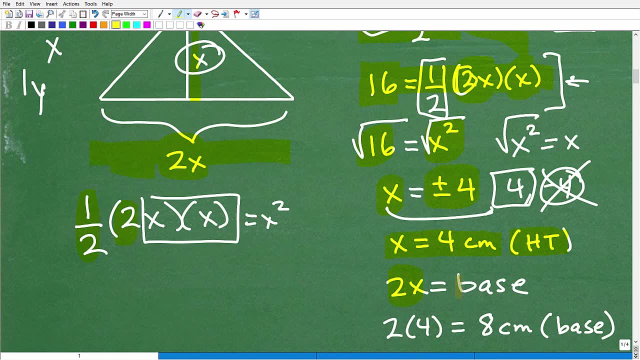 x was the height, And now let's throw in those units of measure, So x is equal to 4 centimeters and the base is twice the height, It's 2x. okay is the base. We know what x is, So I'll just 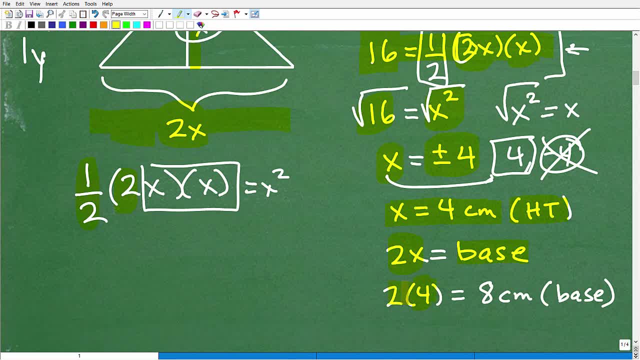 plug in that 4 for x- and I'm going to get 2 times 4- is 8, or 8 centimeters. Remember, in a problem like this, if we're given units of measure which we were centimeters squared for. 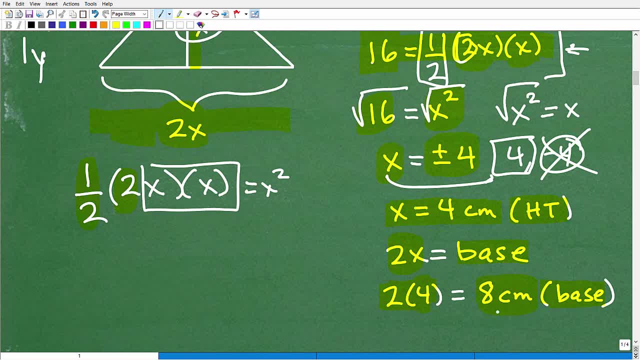 the area and we're asking for the base and the height. that's the length, So 8 centimeters and 4 centimeters. that is the answer. That's the base and the height, And if you got this problem right all by yourself, I must give you a big happy face. 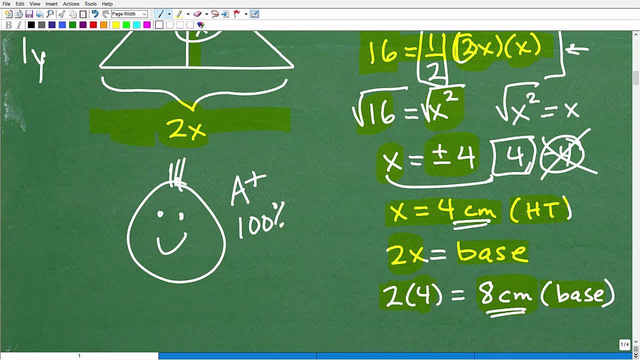 Mohawk an A+, a 100%, And I'll give you two stars as this wasn't the most difficult problem. okay, There's a lot more challenging problems. And listen when you watch my videos. if I give you like four or five stars, that means a problem's difficult. I do have.